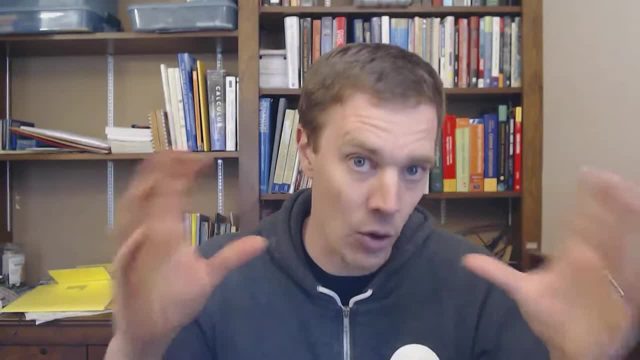 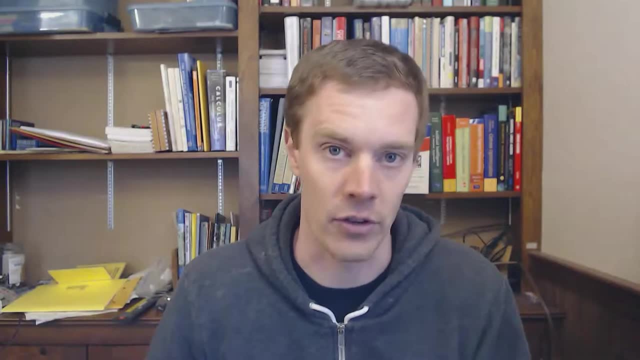 but there's also other techniques as well. And again, so if you can frame your problem, whatever kind of problem it is, if you can frame that as a finite state machine, then suddenly you can take advantage of all of these tools and you have a very 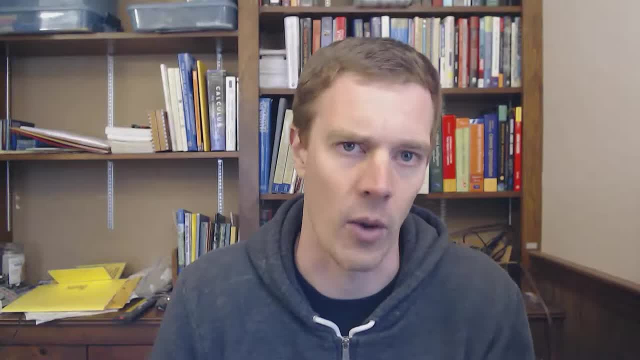 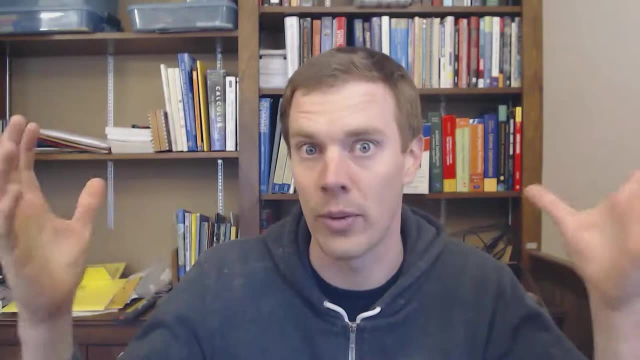 regular structure you can impose on the problem and move forward that way, And if you just try to reason through it with your head very quickly, you're going to get problems that are way too big to fit in your head, And so the finite state machine is this very structured way of working. 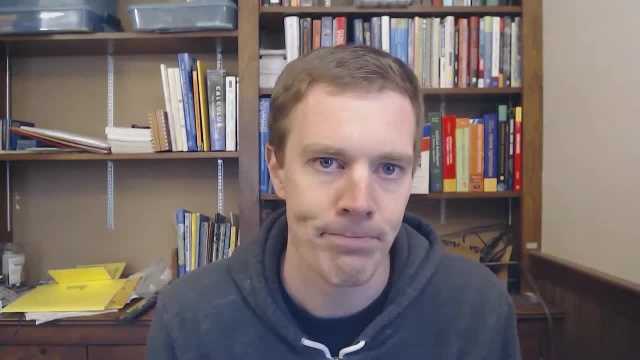 through that problem and turning it into a concrete implementation. So the conceptual structure that we're going to use for our final state machine is a very structured way of working through that problem and turning it into a concrete implementation. So the conceptual structure that we're going to use for our final state machine. 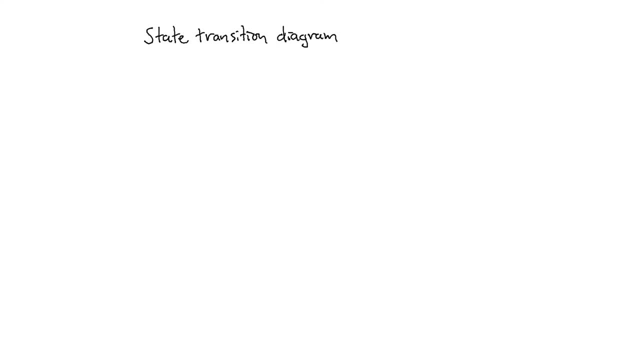 is represented with what we'll call a state transition diagram. So a finite state machine consists of a finite number of states, and in the state transition diagram we'll just create these with circles, And the state machine must be in one of those circles, and then we can define what. 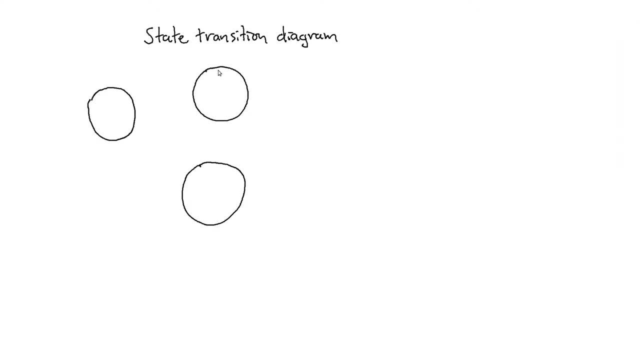 the transition between each of these circles, between each of these states is So, for example, if something happens, if we're in this state and something happens, we receive a particular event or a particular signal goes high or whatever, then we transition to some other state. right, We might. 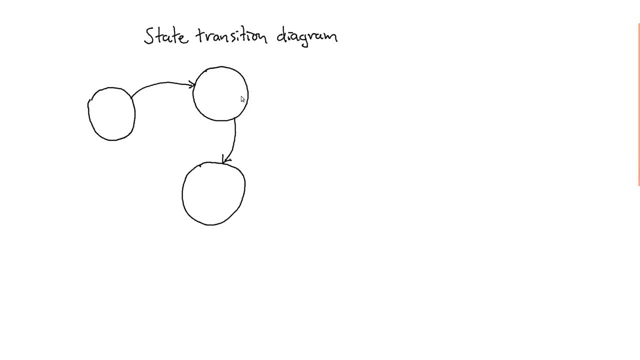 transition from that state to this third state, or if we get a different input, maybe we transition back to the first state and there might even be some other input that we get that we don't actually go anywhere. we just stay in the same state. And so, by drawing out these states, 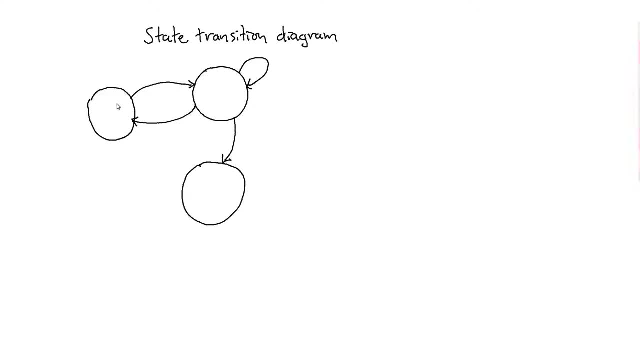 then specifying the transitions between the states. we've completely specified the behavior of this finite state machine. So let's just do a quick example to make this concrete. So suppose I want to build a passcode block, so it's going to have some state that's locked. 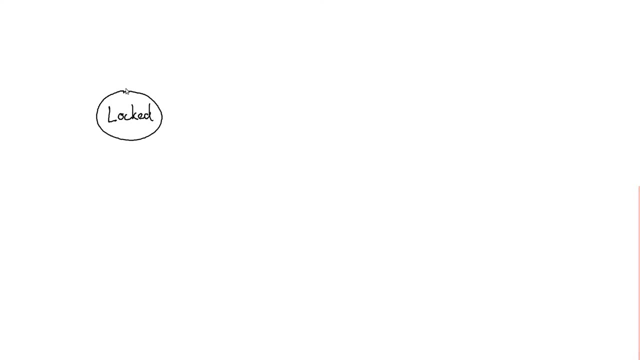 and so we'll circle that that's a defined state, and then there's a state where it's unlocked. that's another state, And if you press, say, a button to lock the system, then it goes from the unlocked state to the locked state. 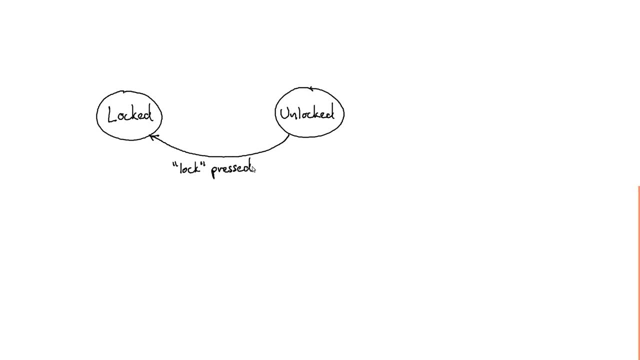 And to go from the locked state to the unlocked state, you're going to need to do a couple things. First of all, you're going to need to do a couple things. First of all, you're going to need to do a couple things. 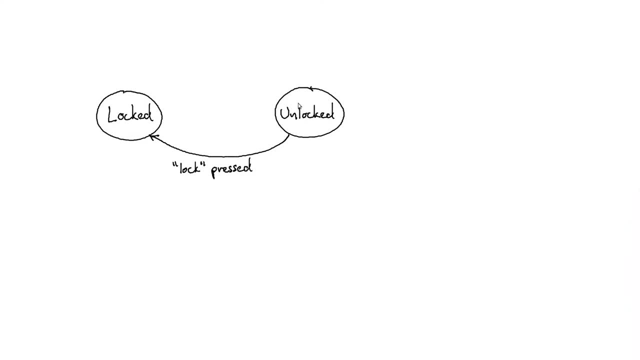 to the unlocked state. you have to enter some kind of passcode And while you're entering the passcode you're sort of neither locked nor unlocked. The lock is still physically closed, but maybe you've got some indicator light or something that turns off. so we might say entering passcode is a separate state here. 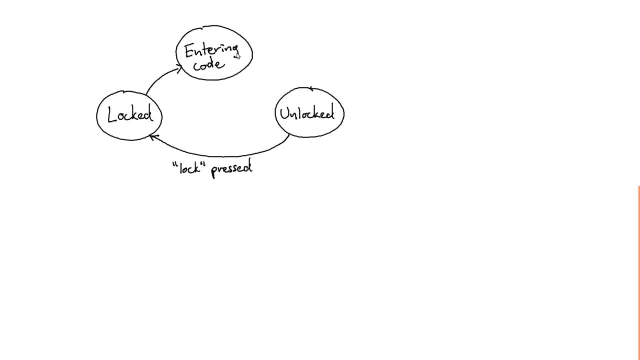 So anytime a code button is pressed, we would move into that entering code state And if we get the correct code, then we would move into the unlock state, and if we got the incorrect code, then we would move back into the lock state and allow the user to. 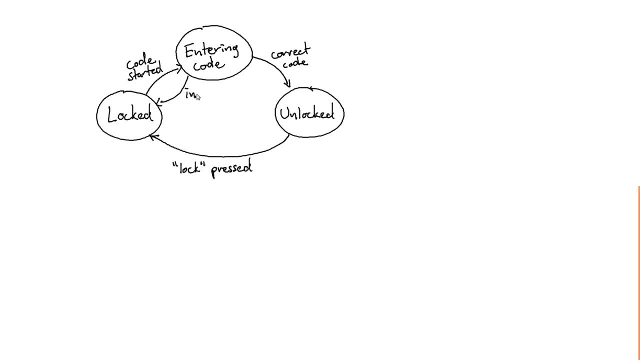 try again with a new code, And so here we've completely specified what could happen in each state. So if you're in the lock state, the only thing you can do is just start punching a code at some point. If you're entering a code, either you get the correct code and you moved into the unlock. 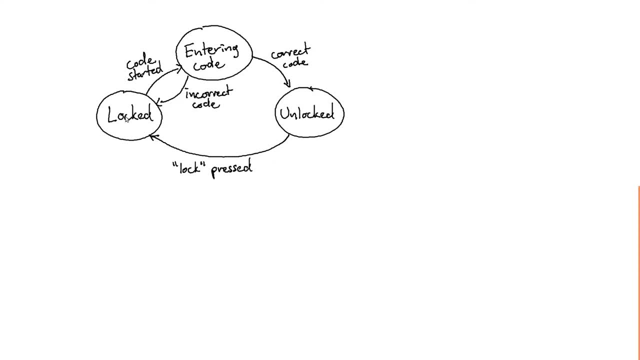 state, or you get an incorrect code and you move back into the lock state when you're in the unlock state. So you just stay there until whatever button is pressed that makes you move back into locked. Now we could also add behavior to each of these states. 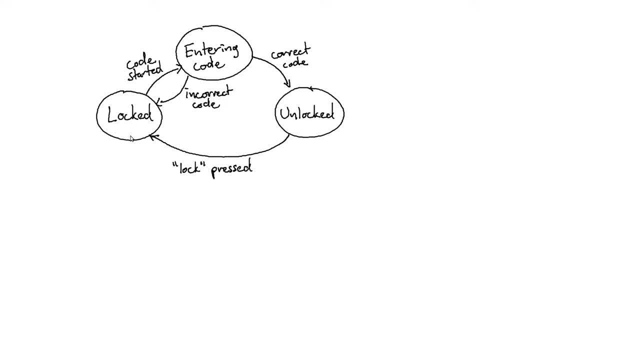 So, for example, we already said that there's a physical lock and we only want to unlock the physical lock when we're in the unlocked state. So in both the locked and entering code states the lock output will be two: We'll be locked and in the unlocked state the lock output is unlocked. 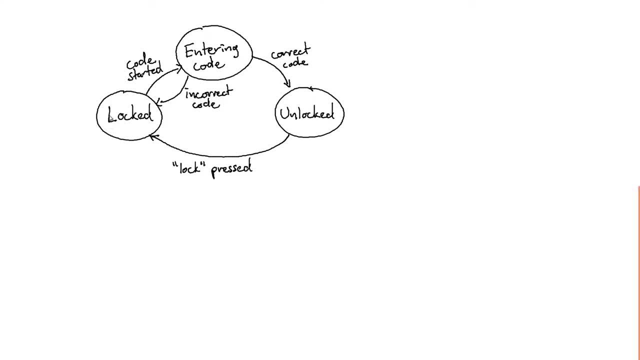 We might also have LEDs or some kind of indicator that says enter a code when you're in the locked state, but not once you've started entering the code. maybe that light goes off, or something like that, And so we can define output variables or output behavior in terms of which state the system. 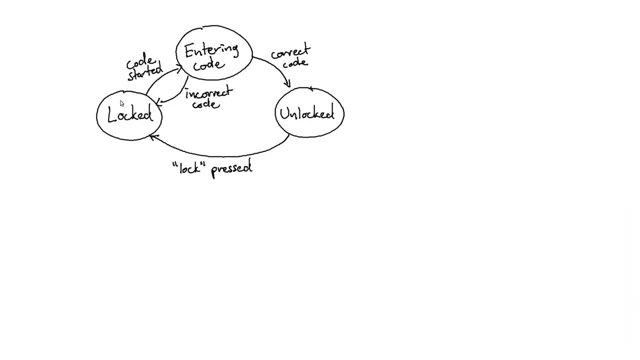 is currently in. Okay, So that's it. Thank you, Bye, Bye. So that's the conceptual structure of a finite state machine. Let's talk about how we would actually implement this in hardware. So the hardware implementation for a finite state machine. the core piece is: we've got 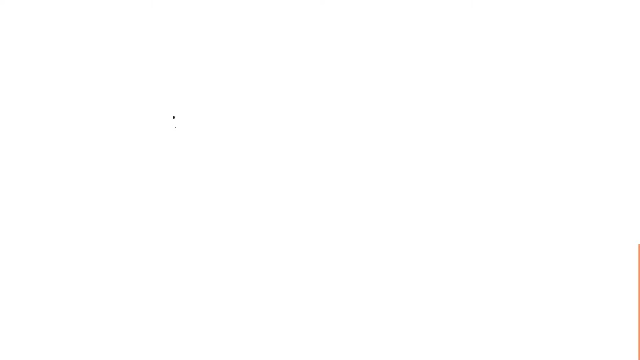 some kind of thing that holds the actual state, And so that's going to be a register, and again, a register in this sense just means a bank of flip-flops. So I'll just draw this as two flip-flops here, although it could just be one flip-flop could. 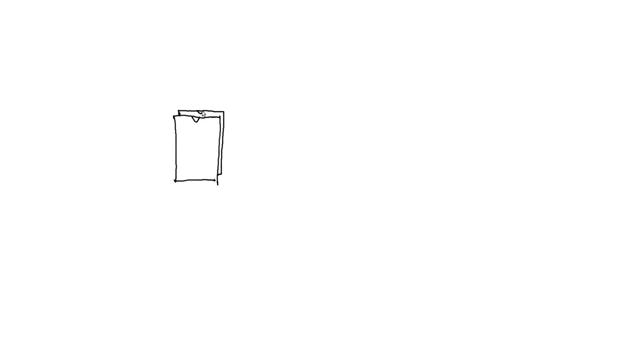 be two, could be any number of flip-flops stacked up together. Okay, Then we've got some logic, that, and so coming out of here, we've got some representation of the current state, and then somehow we need to take the current state and whatever. 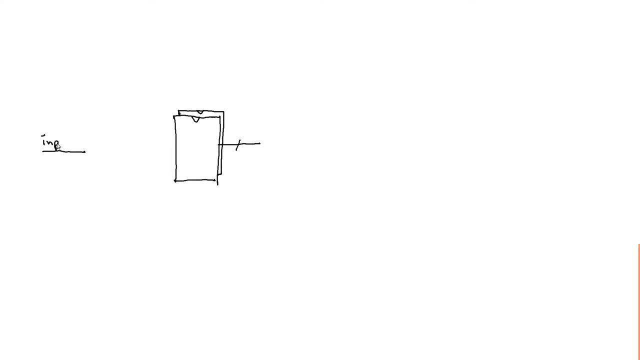 the current inputs are. so some inputs and combine those to figure out where we're going, what the next state is. Okay, And so we're going to create some kind of nebulous blob of combinational logic here. We'll call this next state logic, because this is logic that is going to again take. 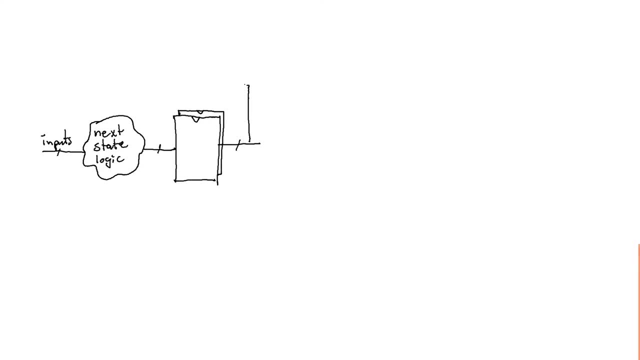 the inputs. take the current state here and compute whatever the next state of the system should be. Then we've got our current state, Okay, So we're going to use that to compute some outputs here, and the outputs again are: 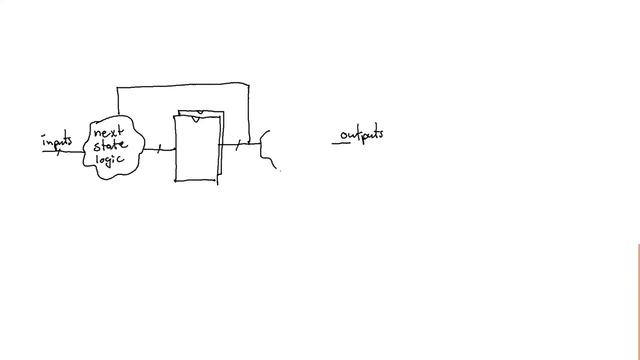 some function of the current state. So we'll call this nebulous blob of combinational logic the output logic. This is one basic design pattern for implementing a finite state machine in hardware. It turns out there's actually another pattern. So if we design the finite state machine slightly differently, we can actually add another arrow. 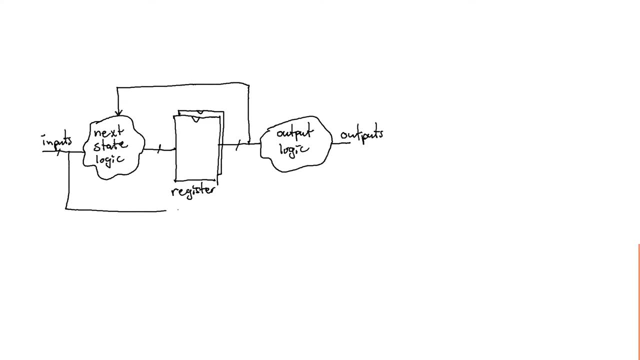 saying that if we take these inputs here and we actually use the inputs as an input to compute the outputs, so we've kind of got this shortcut for the inputs to affect the outputs directly into this output logic here. that would create a Mealy machine. 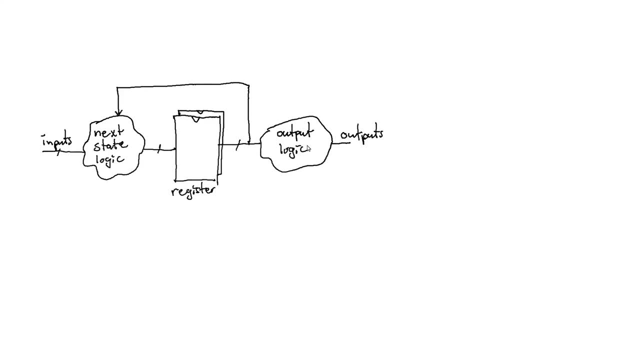 And the design here that we've shown so far is what's known as a Moore state machine. At the end of this video series, I'll have a video that describes the difference between Mealy and Moore and when you might use one or the other. 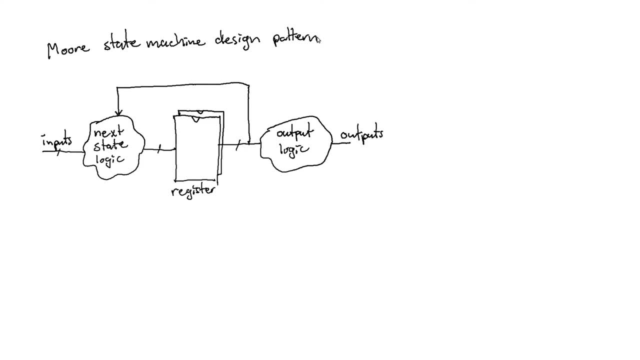 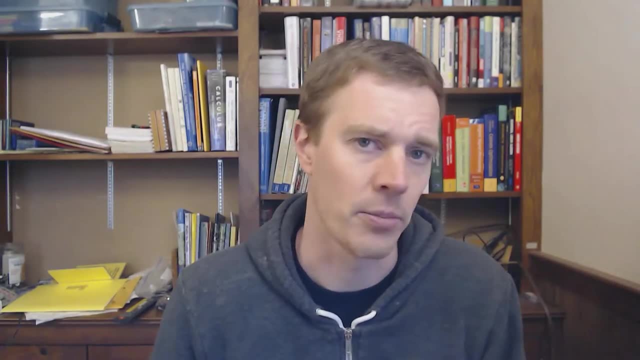 But for now just focus on understanding how a Moore state machine works. A common question that comes up is: like: do I actually need to build finite state machines, or is this just kind of some curiosity as we're going through the course? Absolutely, you need to be able to build finite state machines. 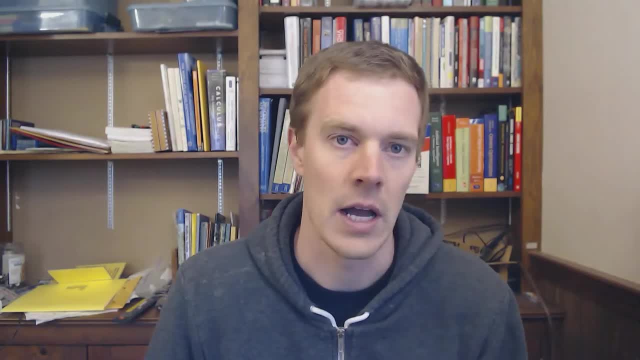 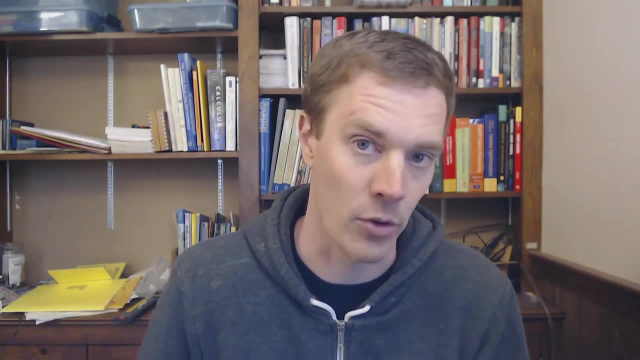 So sequential logic, everything we've talked about so far: counters, shift registers, memories, all of those things you can think about conceptually as a finite state machine. It may not be the most helpful representation, but I think it helps to make that link. 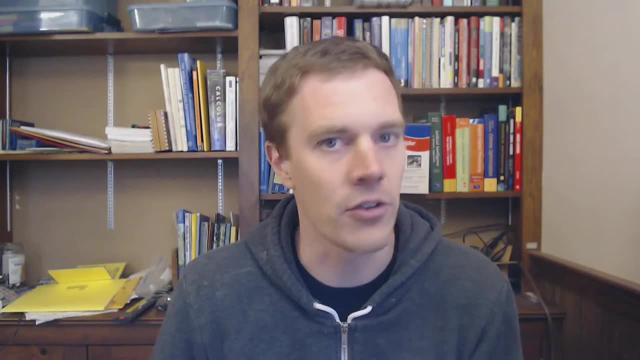 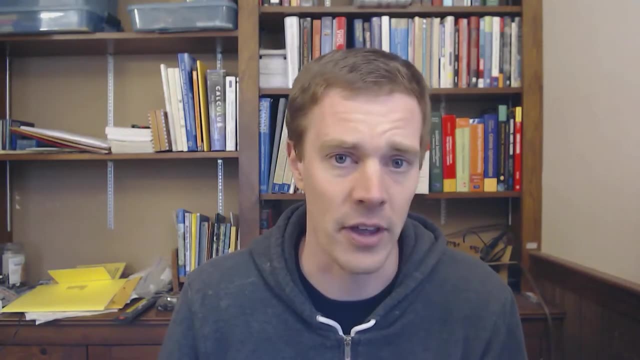 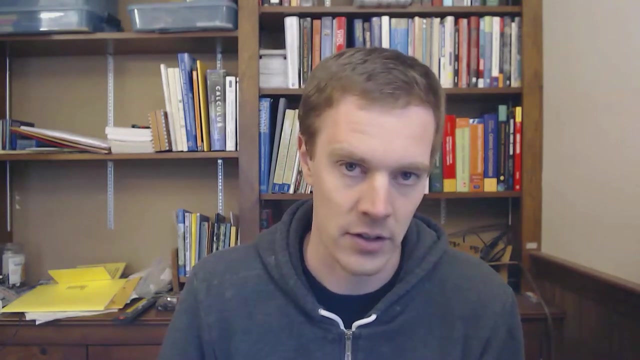 Okay, And then if you want any sort of complex decision-making behavior, that's almost certainly going to be a finite state machine. So in fact we've already built lots of things that are state machines. So if you could think about a binary counter as a state machine, in the sense that every 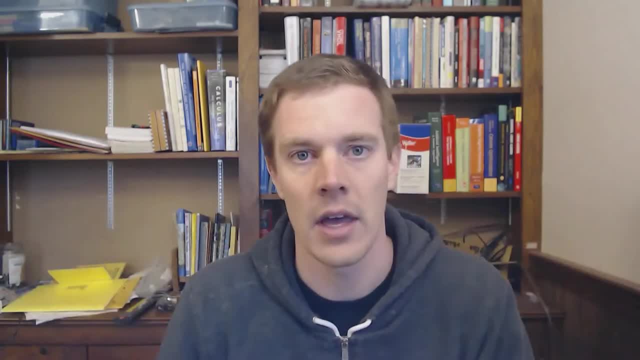 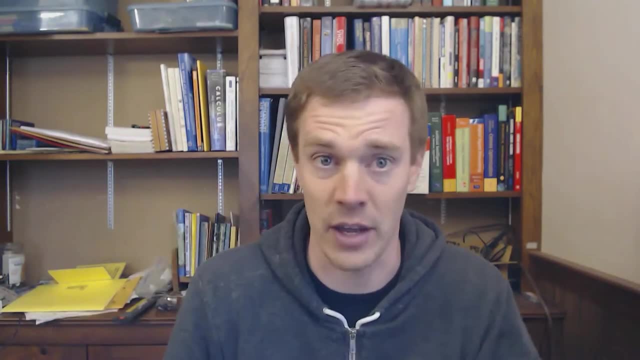 sequence of bits that it produces is a state and it has regular transitions from one state to the next that occur on every clock cycle. it doesn't necessarily have any inputs, or it might have an input. It might have a count or a don't count, or a count up or a count down that add more. 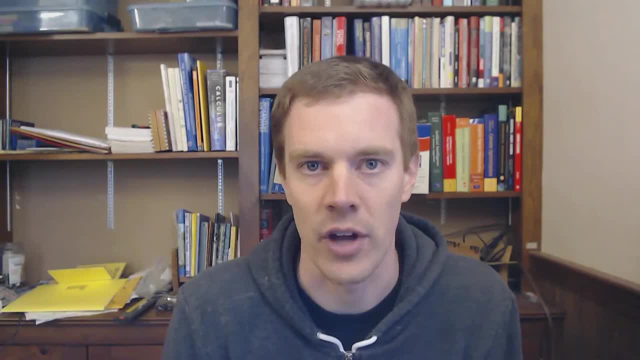 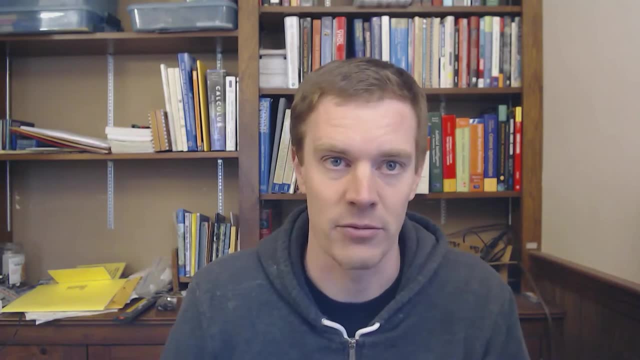 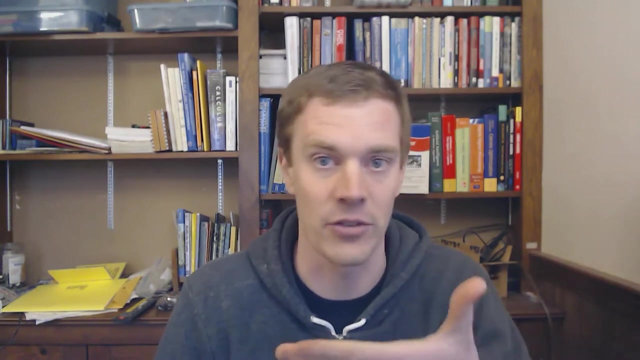 decision-making behavior more edges to its state transition diagram, Something like a two-bit shift register. again is a finite state machine. It's got four potential states with all of the possible combinations of ones and zeros coming out of the shift register and it changes states based on what's coming in to the FSM. 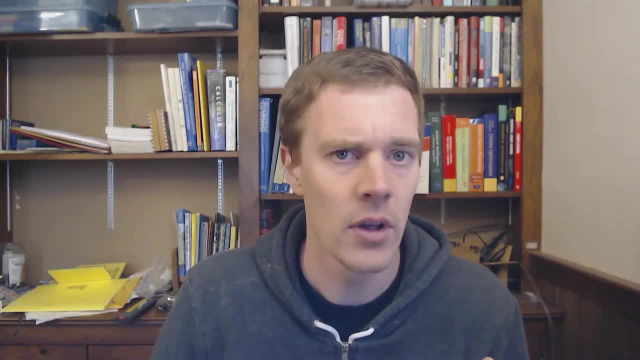 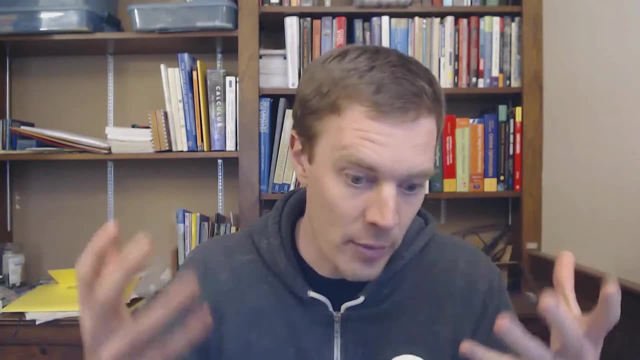 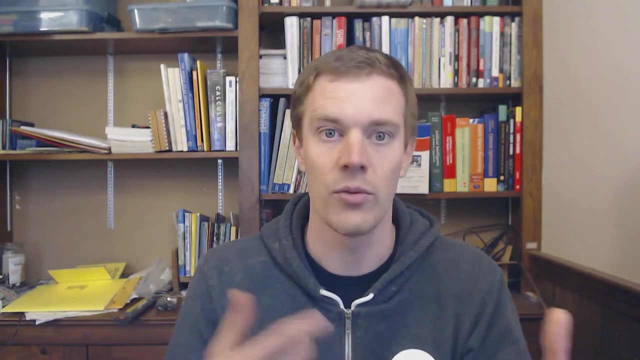 So again with these, it's probably not helpful To think of them primarily as state machines, But I think, making that mental link, that you could think about any digital circuit as a finite state machine, any digital circuit that has some state, and that state can evolve.